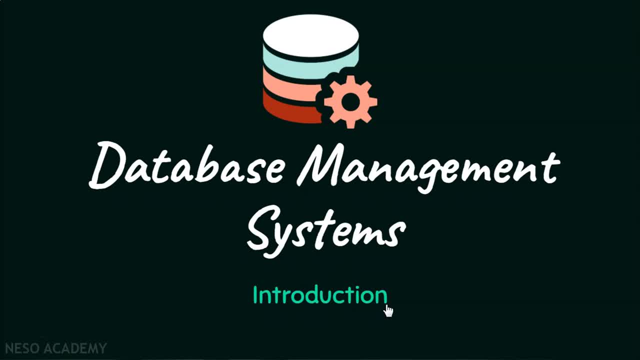 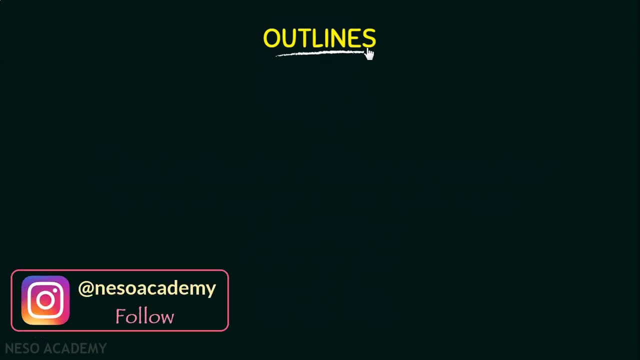 more about file systems and why we prefer DBMS approach over the file system approach. Before we get into the topic, let us see the outlines, or the topics that we are going to cover in this video. The first one we are going to see is the basic definitions, or the 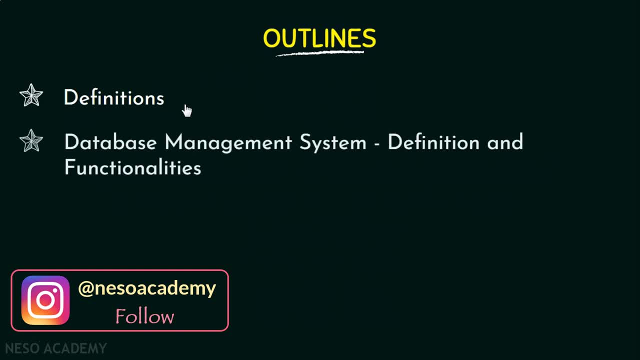 basic terminologies that we need to know. Next, we will be looking into the definition and functionalities of database management system, and then we will be discussing about the properties of database. Next, we will be briefly looking into an illustration of a simplified database system environment. 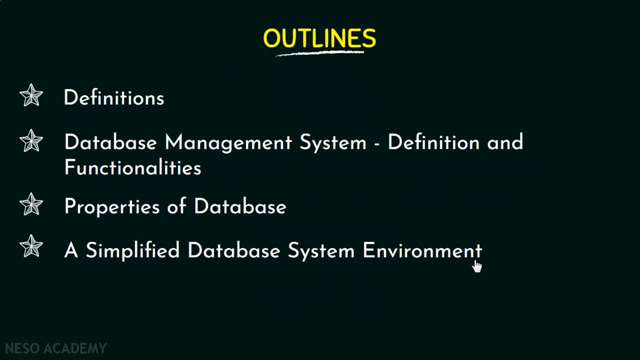 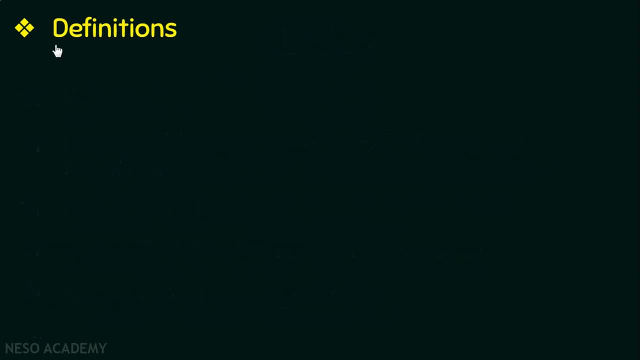 and then, finally, to understand database and its functionalities better. we will be looking into an example of a university database. So, as we discussed, first, we will be looking into the basic definitions in relation to DBMS. The first one is data. Data is any raw facts or unprocessed facts that you can record. 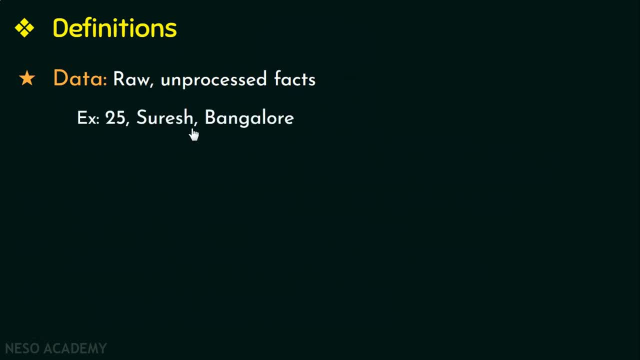 Like, for example, any numbers, name of a person, name of a place, any kind of text, images, audio video, etc. all these are called as data. Next, what is information, These unprocessed facts or otherwise called as data, when they? 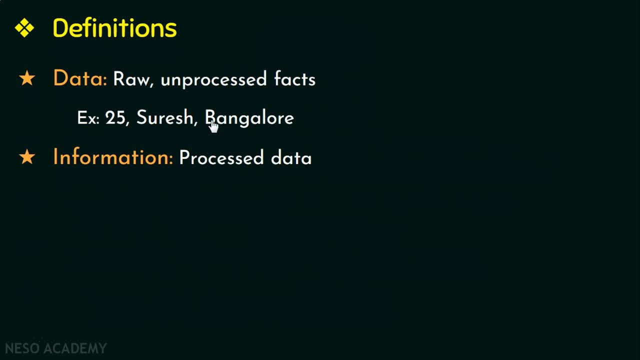 are processed to make a meaningful context, then that is called as information, or in other words I can say it is the processed data, data like, for example, the age of Suresh is 25. so here I take the raw facts or the unprocessed facts, process it to make a meaningful context and that is called 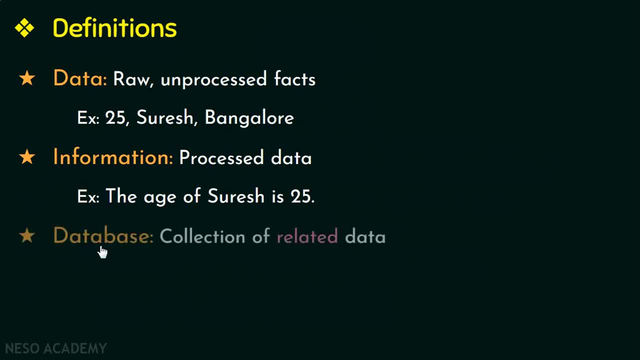 as information. next, let us see what is a database. database is a collection of related data. now, a random collection of data or data that is not related cannot be referred to as a database. it has to be a collection of related data, like, for example, the data in an online banking system database has to be related to. 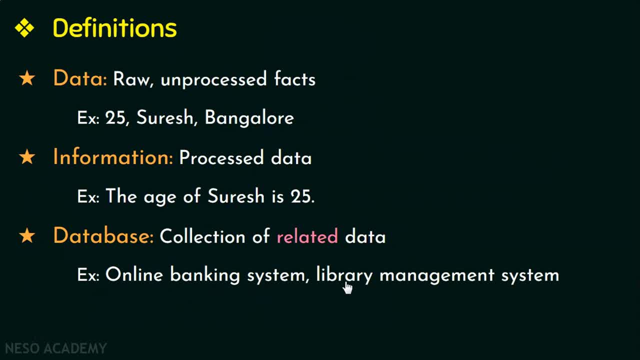 that particular bank. similarly, the data in library management system database has to be related to that particular library. so this is what we call as a database. the next one is metadata. metadata is necessary in order to create a database. the database of data is very important. nothing but the database definition, or in other words, I can say it is the complete description. 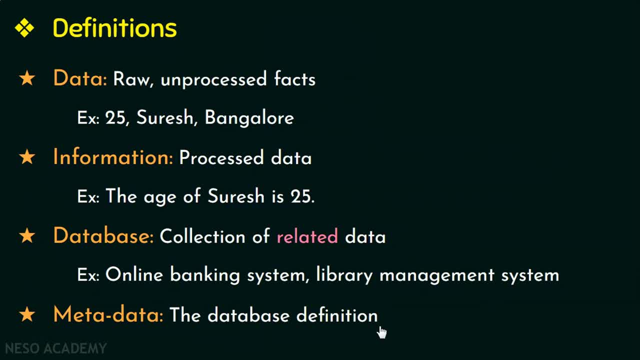 of a database or it defines the database Information, like the storage format or the data type of the data that we are going to store in the database, or the constraints on the data. all these information is called as metadata. So these are the basic definitions we have seen. 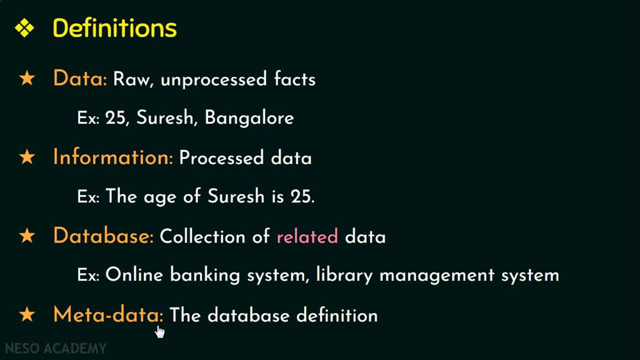 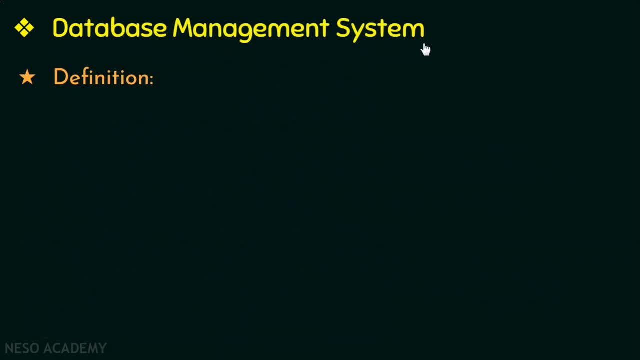 In the further videos we will see more definitions in relation to DBMS. Next, let us see the definition of database management system. Database management system is a system to manage the database, and here managing could be either storing of data or retrieval of data from the database. Now let's 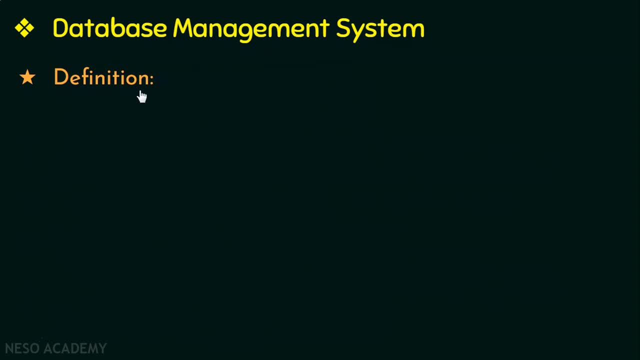 look into the proper definition of database management system. Database management system is a system or database management system that is used to manage the database. So database management is a software, or I can say it is a collection of programs that enables users or that allows the 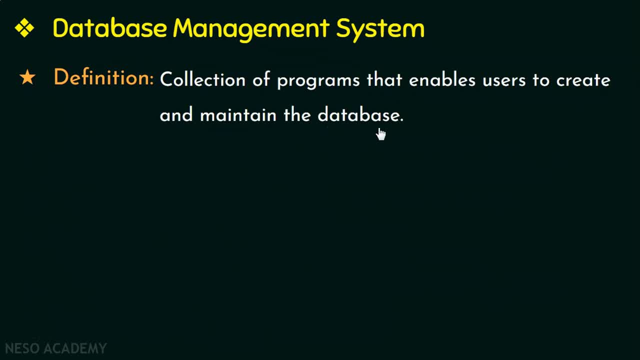 users to create and maintain the database. So this is a very simple definition. Now let's move on to the functionalities of database management system. Database management system allows users to define the database, to construct the database, manipulate and manage the database. So database management. 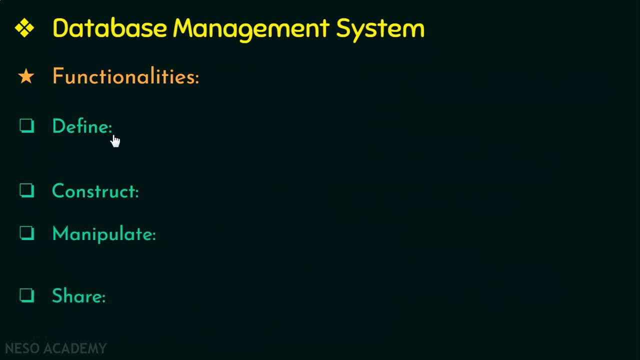 system is a system that allows users to share and manage the database. Now, defining the database involves specifying the data type for the data that we are going to store in the database. also specifying the structures and constraints for the data- Now constraints- is nothing but the. 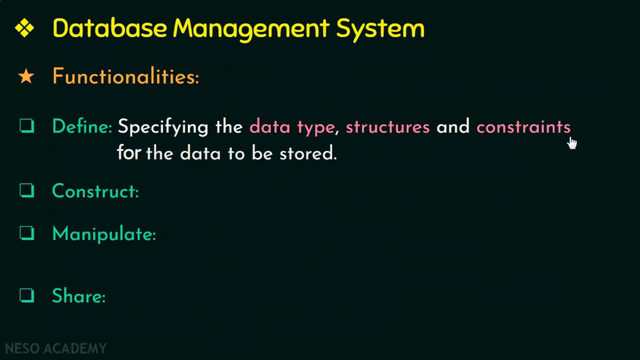 limits on the data, Like, for example, if I have age as the data to be stored, then I can have a constraint, say age greater than 18.. So only if age is greater than 18, then only that data can be stored in the database. 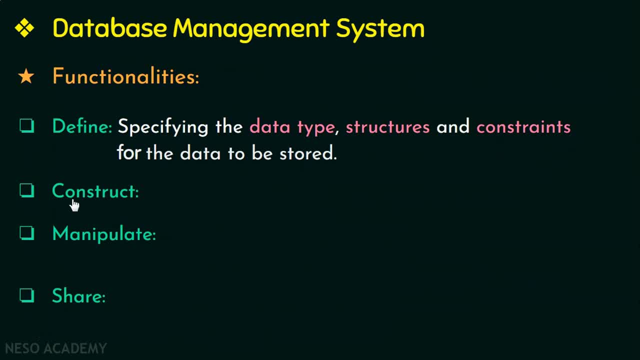 So that is what we call as a constraint. The next functionality, constructing the database, is nothing but the process of storing data on some storage medium, Or in other words, I can say it is the storage of data. So when data is stored, a database is being constructed. 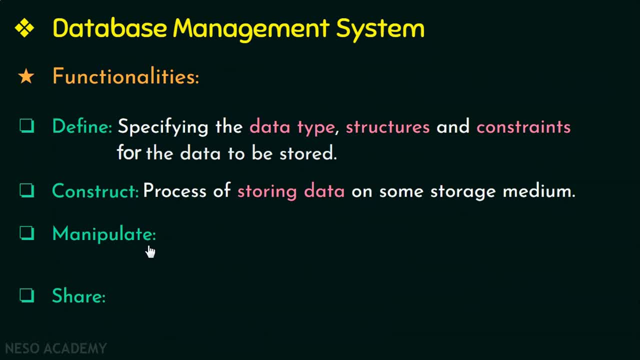 The next functionality, manipulation of a database, includes functions like querying the database to retrieve or to get any data that the user needs. It also allows users to update the database and for generating reports. The next functionality- sharing the database- allows multiple users and programs. 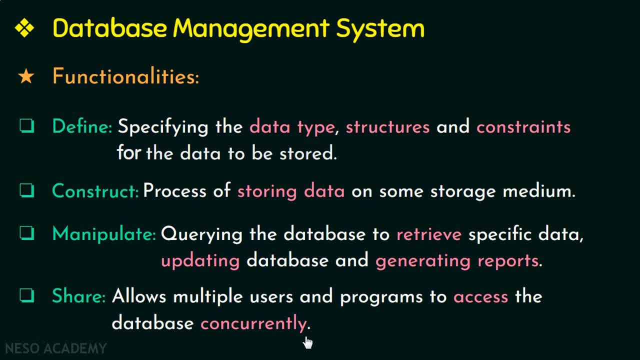 to access the database concurrently or simultaneously, Or in other words, I can say many users can access or share the same database at the same time in an efficient manner. So these are the main functionalities that DBMS provides. The other functions provided by DBMS are protection. 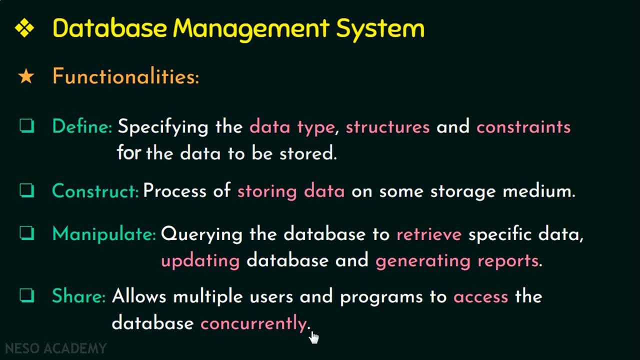 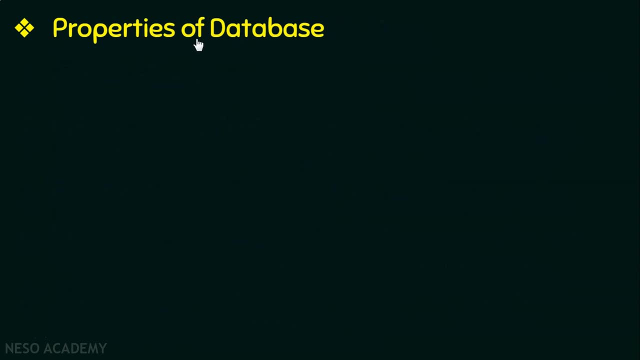 of the database from unauthorized access or from hardware or software failures, and also maintenance of the database for a long period of time. So that is with the functionalities of database management system. Next we will be discussing the properties of database. There are three properties of database. 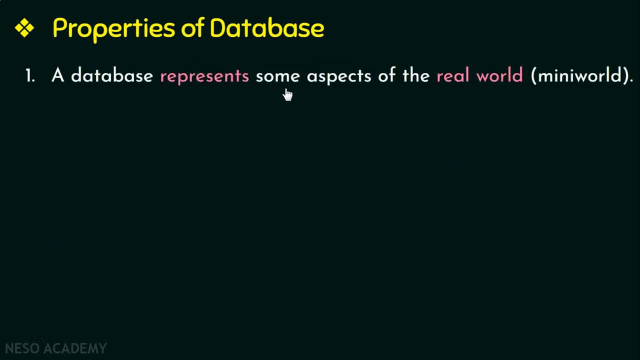 The first one is the database management system. The second one is a database. represents some aspects of the real world, or otherwise called as the mini world. So anything in this mini world, the objects, their properties, the relationships between them, all that is represented by a database. 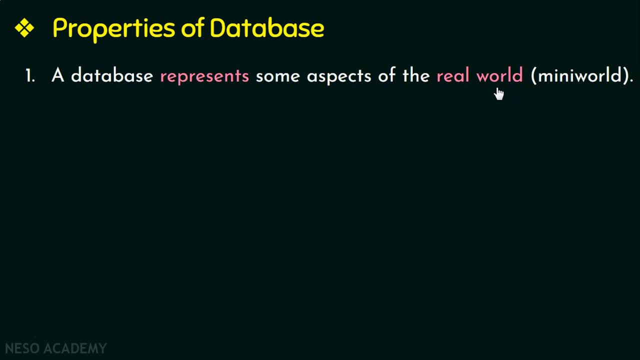 And if there is any change in the real world, that change will also be reflected in the database. The second property is: a database is a logically coherent collection of data with some inherent meaning. So, as I said earlier, a random collection of data or unrelated data cannot be referred to as a database. 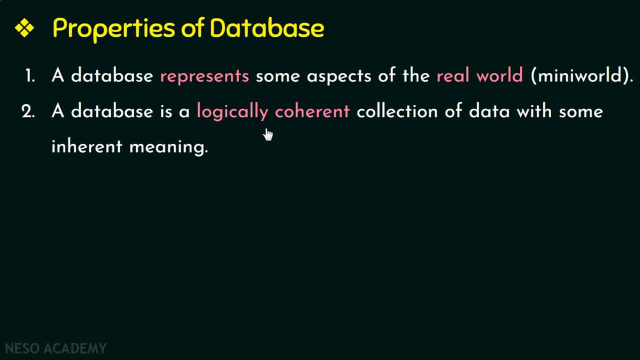 The data in the database has to be related or logically coherent. The next property is: a database is designed and then built and populated with data for a specific purpose. So these are the three main properties of database. The first one is: a database represents the real world. 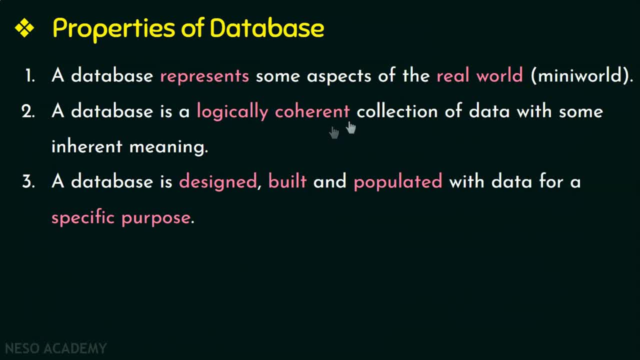 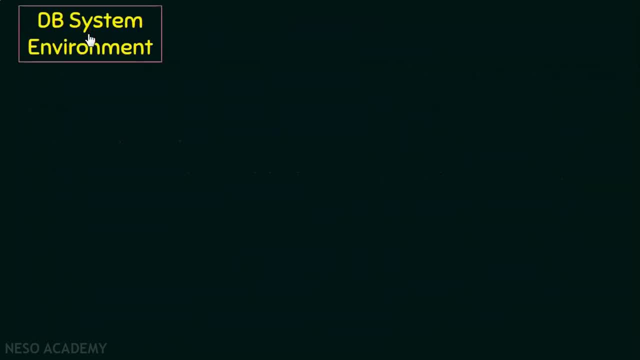 Secondly, it is a logically coherent collection of data. And thirdly, a database is designed, built and then filled with data for some purpose. Next, let us look into an illustration of database system environment. So here we have the users or the programmers. 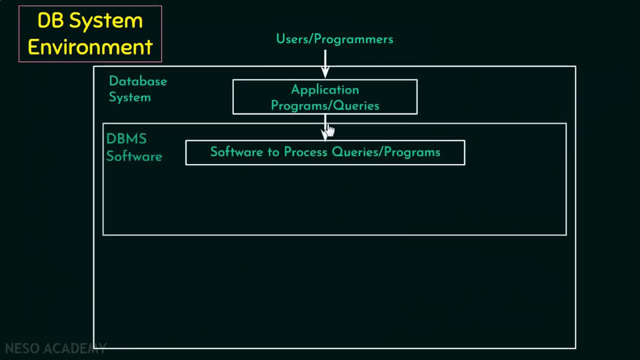 who writes queries or programs, And these queries or programs are processed by the DBMS software And then, based on the processed queries, DBMS software accesses the stored data in the database. That is, it accesses the stored database as well as it accesses the metadata. 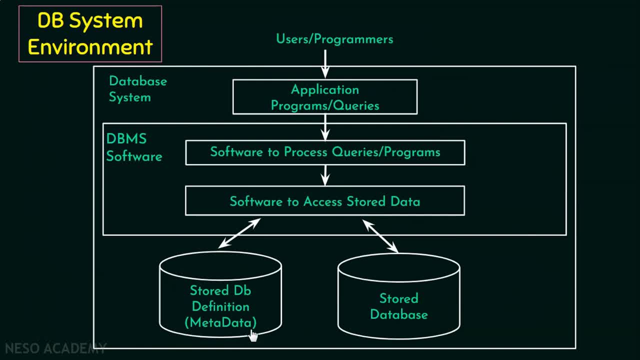 As we have already seen, metadata is the database definition, So this is a simple illustration of a database system environment where users write their queries and it is processed by the DBMS software And, based on the processed queries, DBMS software accesses the stored database. 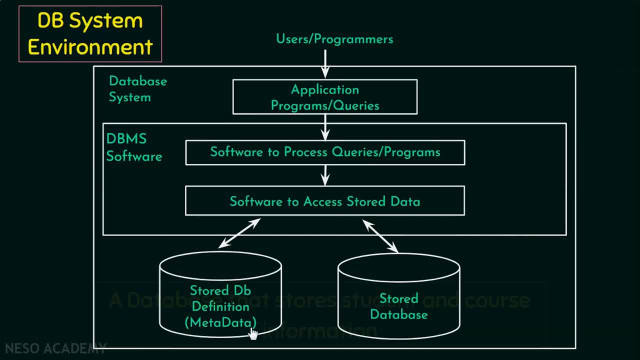 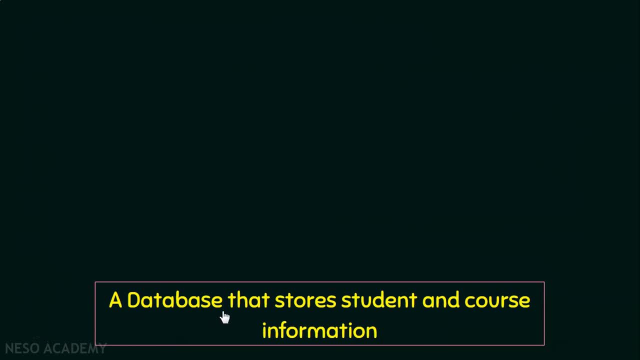 as well as the metadata, As we discussed in the outlines. finally, to understand our database and its functionalities better, we'll be taking an example of a university database that stores student and course information. So here I've taken three tables. The first one is the student table. 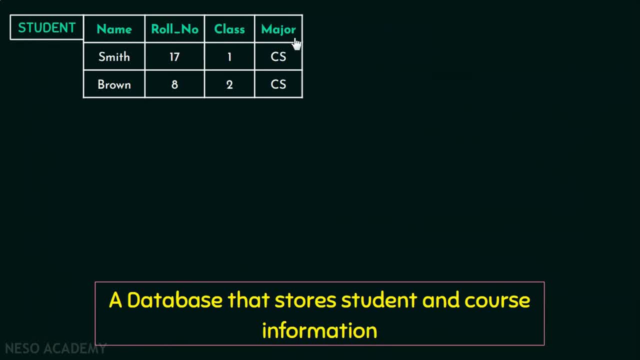 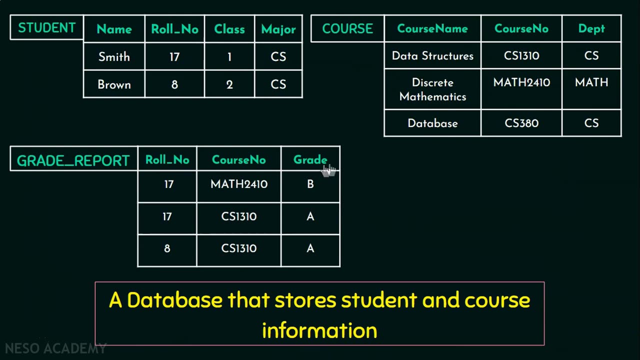 which holds information about the students in that university. The second table is the course table, which holds information about the courses available. And third table is a grade report table, which contains information about the grades received by each student in a particular course. as we have seen earlier, the four functionalities provided by dbms, let us try. 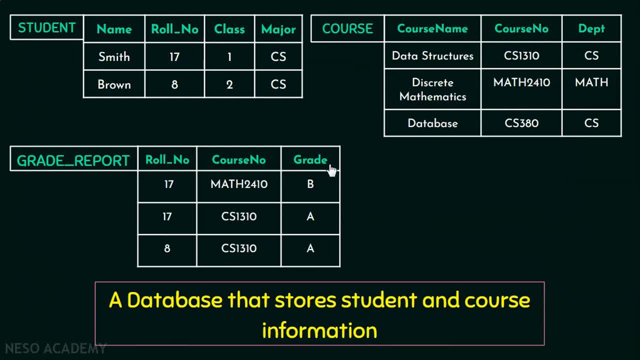 to understand those functionalities better with this example, as we learn, defining the database involves specifying the data type, structures and constraints for the data that we are going to store in the database. so here, specifying the structure of each record means specifying the different types of data elements present in that particular record. so here we have three records. 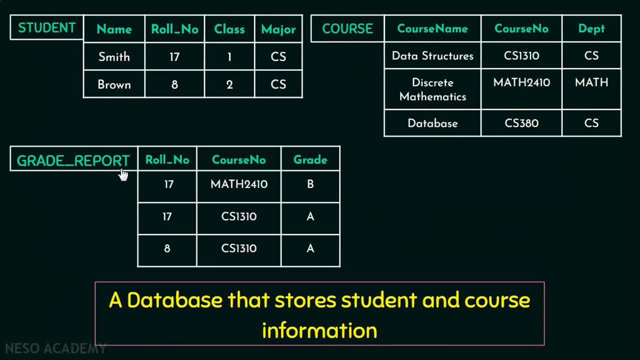 the student record, the course record and the grade report record, and these columns are called as data elements in each record. now specifying a data type would be now, for example, for student name, i can say the data type should be a string of characters, or for data element role number, i can say the data.